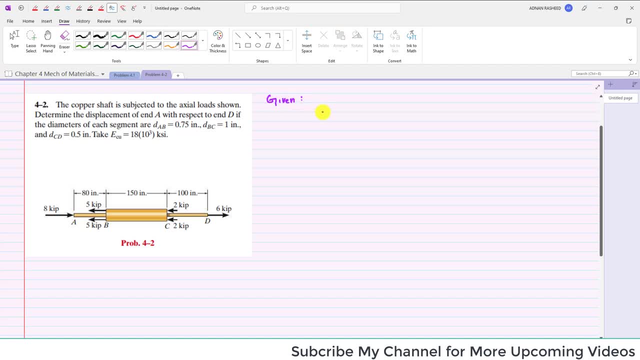 from given data. In given data it is given that E of copper is equal to 18 into 10 to the power 3 KSI. Clear diameter of rod AB DAB is given as 0.75 inch D of BC is equal. 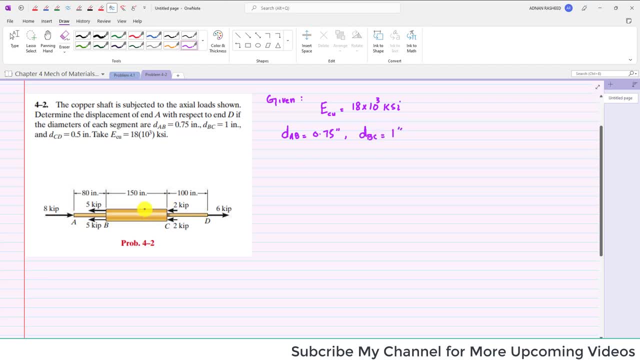 to 1 inch. This is D, This is DAB, DBC, And D of CD is equal to 0.5 inch. So what we have to find is that displacement of point A with respect to point D. So I will write it: displacement of point A with respect to. 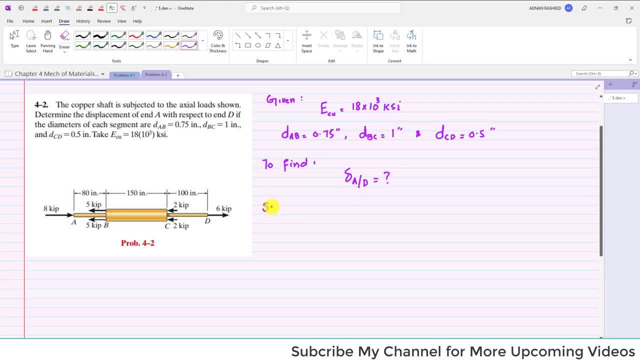 point D. We have to find this clear. So first we will find the displacement in each rod or AB, rod BC and or CD. So for that I have to first cut the rod AB over any point along the length of AB. So if I cut rod AB at any point, So this is D, This is A and this is B at any point. So at 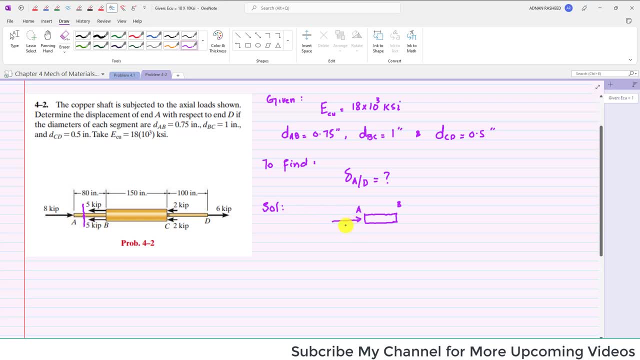 the end of rod A we have a load that is given as 8 kips, And if I cut it at any length in order to keep it in equilibrium there, this load will be equal to PAB, And this is from simple calculation. This is again equal to 8 kips. Now we will cut the rod BC at this. 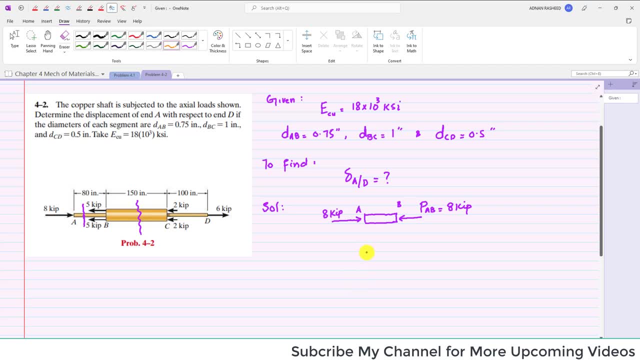 point. I will use another color. So this is having larger diameter. and this is rod AB. Clear at A point this load is 8 kips. This is point A, This is point B. So at point B there are two loads, that is, 5 kips and 5 kips. So now you can add them, These two rods. 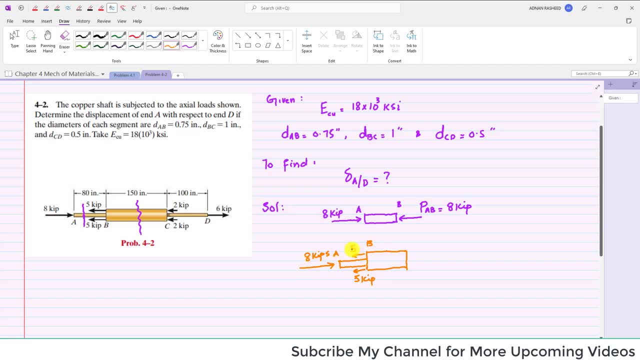 are in on left side and this force is on right side, So this is 10 and this is 8.. So we need 2 force in order to keep in equilibrium. So I will write here: this PBC will be equal to 2 kips Because it will keep if you apply 2 kips at this point. So this will be in equilibrium. 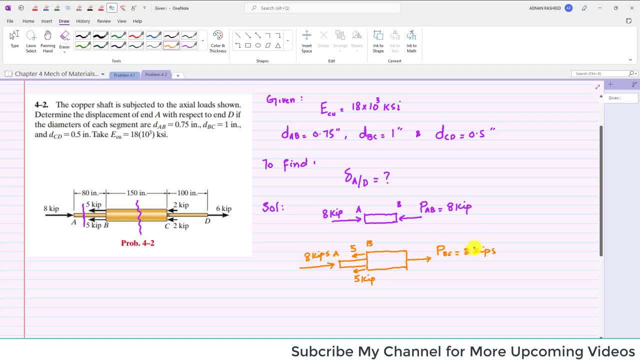 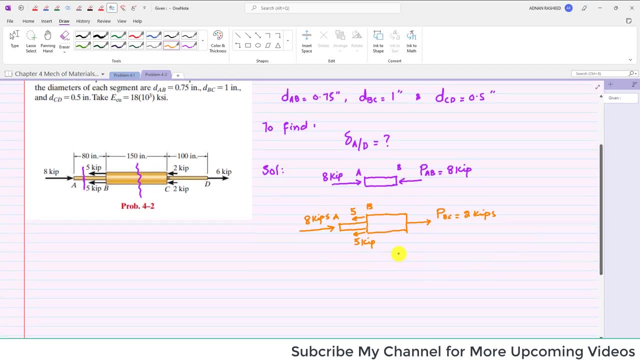 because you can see 8 plus 2 is 10 in right side, while this 5 plus 5 on left side, So it will keep it in equilibrium. So from here we can get: PBC is equal to PBC. So this is. 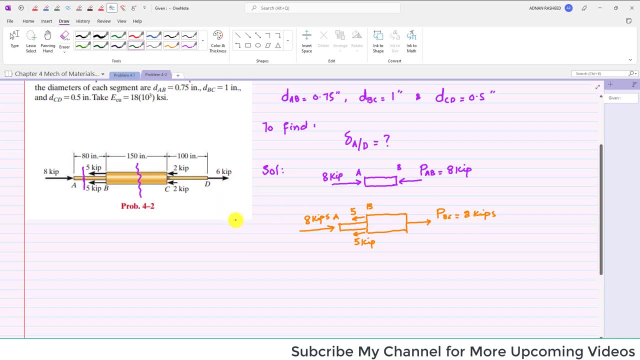 equal to 2 kN. Now I will apply. I will cut the third portion of the rod, which is this: So if I cut it and take it from the right side, So you will see that at this, and this is 6 kips Kips Clear. So, in order to keep it in equilibrium, PCD will be equal to again. 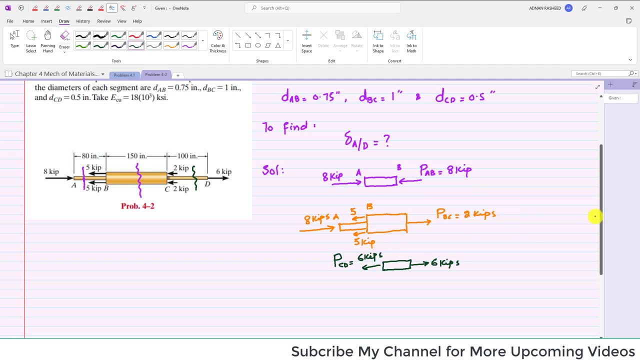 6. Now we will find the displacement of point A with respect to point C, And we know that displacement is equal to PL divided by AE, And if there are more than one segment, so we will write summation. So starting from the first rod, So you can see here the load. 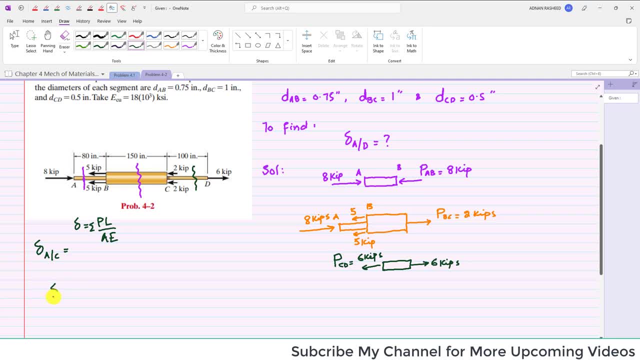 is in compression, So I will write displacement of rod A with point A with respect to point D, not C. This is point D, Clear. So displacement in this rod. this, since this is in compression, So I will write P is minus 8.. Length of this rod is 80 inch. So 8 into 80 divided by area, Area of this rod diameter. 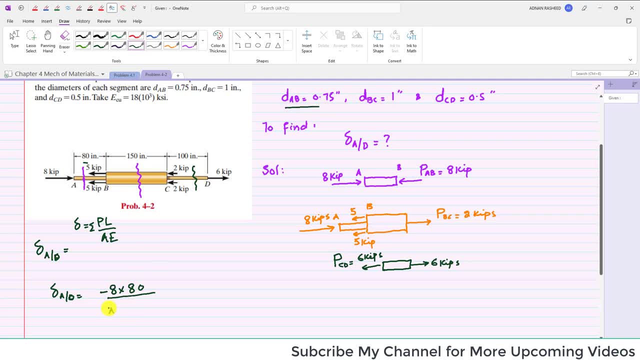 is given. So area will be equal to pi by 4 into 0.75. whole square multiplied by E, and E is 18 into 10 to the power 3.. 18 into 10 to the power 3.. Clear Plus displacement in rod or elongation in rod. BC. Now load in.